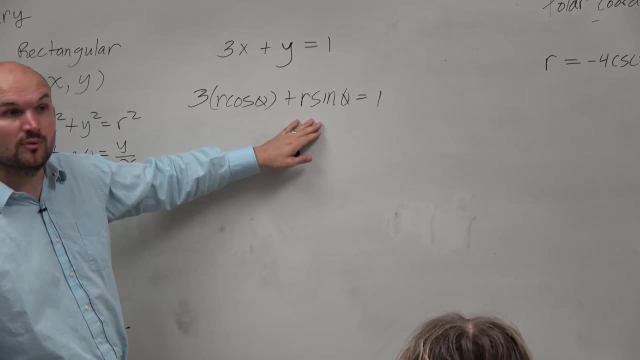 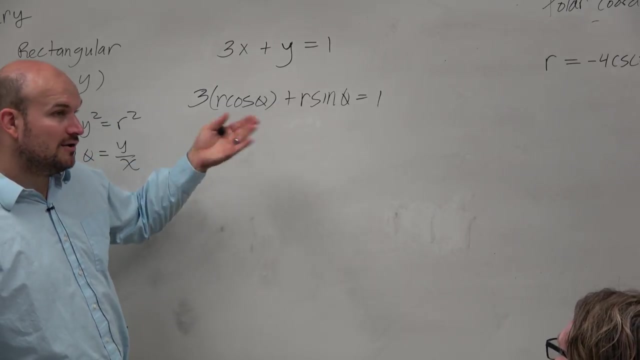 Does that make sense, though? I'm just substituting in x and y for what they represent in polar form. And then now, if we want to write a polar equation, just like when we write rectangular equations, we want to solve for y usually, if we're allowed. 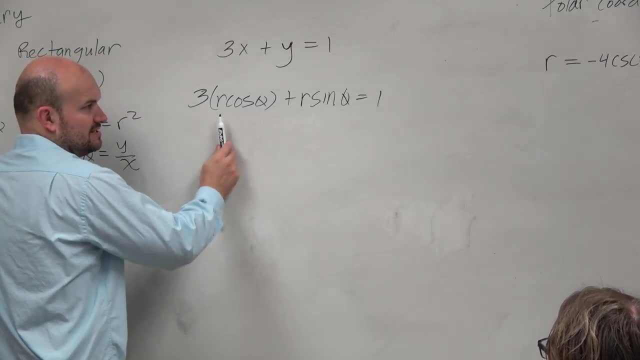 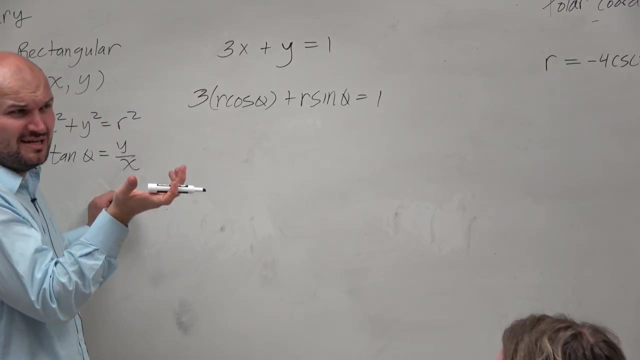 Here we want to solve for r, So should we combine these? Can we combine like: what's cosine plus sine? Is that like tangent or something? Or can we do that? Are those like terms? They're both trig, but they're not like terms, guys. 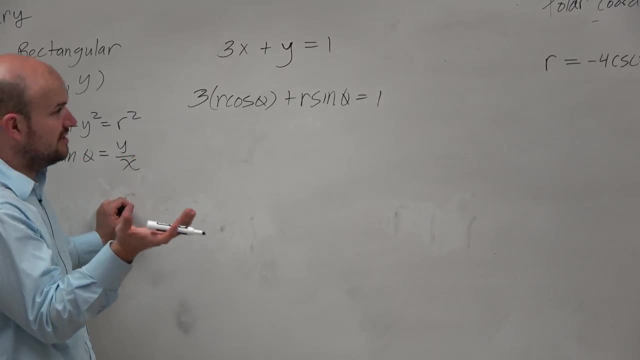 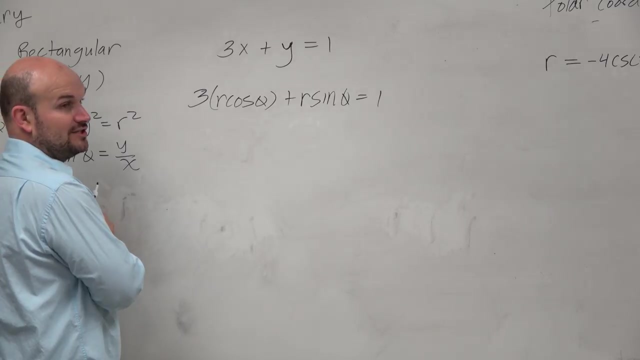 OK, That's like saying x and y, they're both variables, just come out. No, they're not the same. So if we can't combine them, we could maybe rhyme use with a tractor. and it starts with an f. 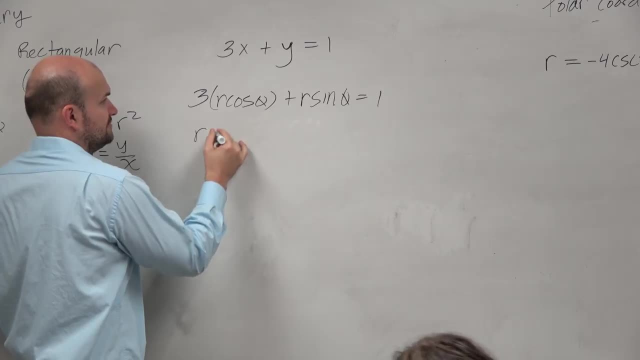 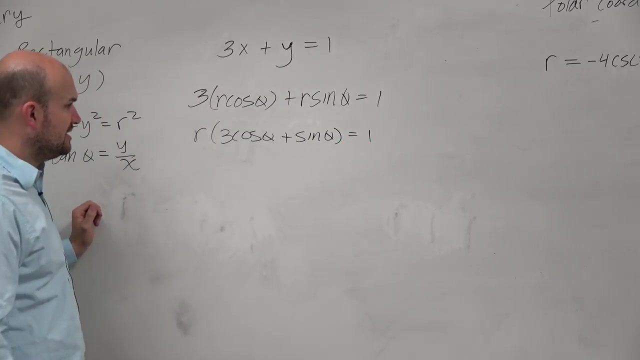 Factor. Can we factor out an r? We could factor out an r. Factor out an r. we're left with 3 cosine theta plus sine of theta. Now going back to algebra, one days, if you want to solve for r. 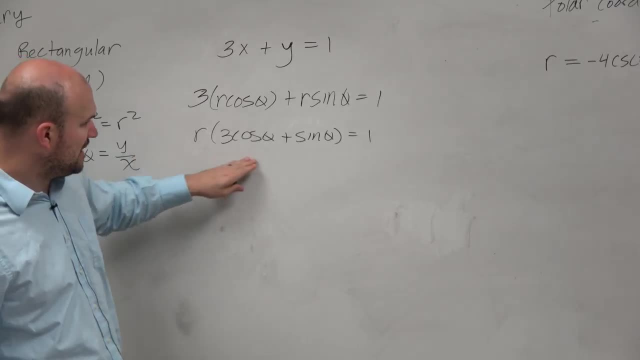 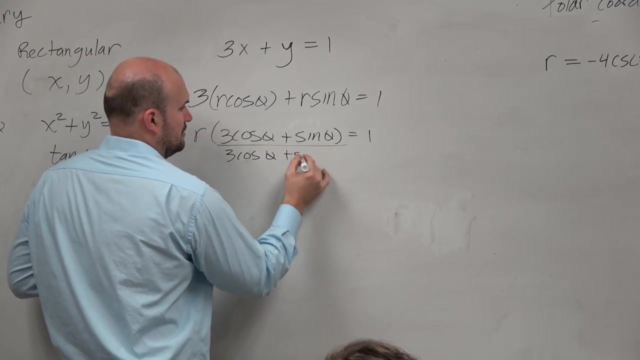 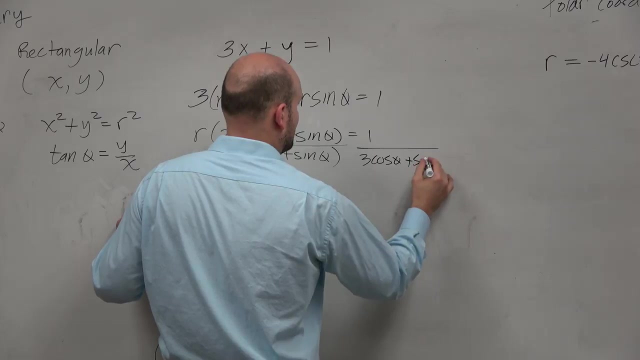 apply the inverse operation. what's being applied to r? Well, r is being multiplied by this quantity, So therefore we just need to divide by that quantity on both sides, And I'm going to waste a lot of ink writing this whole thing out. 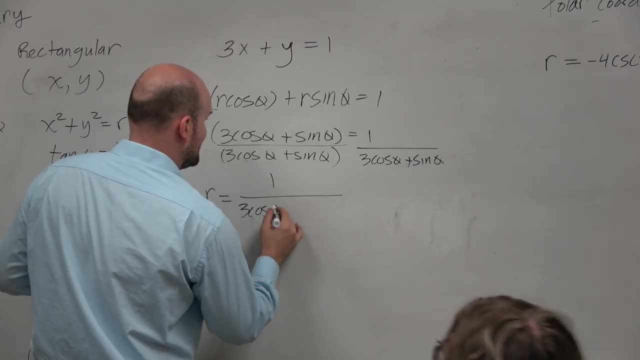 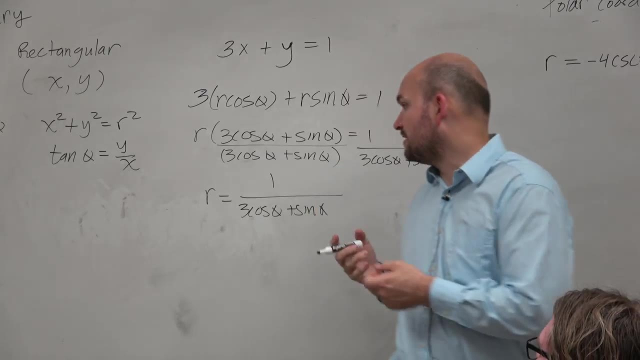 So r equals 1 over 3 cosine of theta plus sine of theta. And what the cool thing is, next class period. I don't have time today, But next class period. what I'll do is we'll plug this in our calculator. 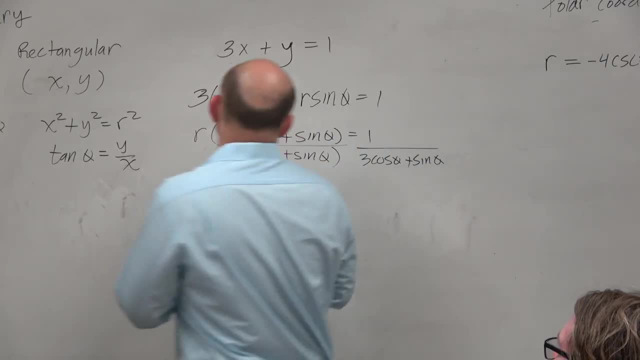 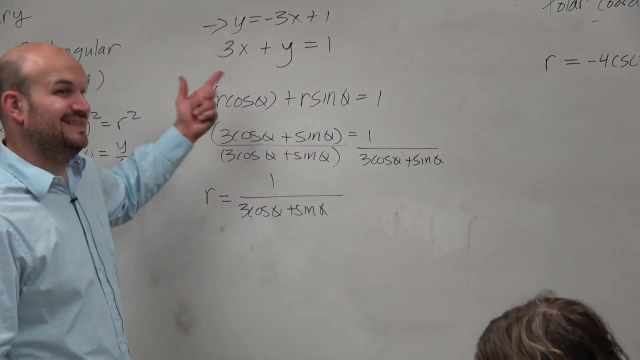 And you guys will see, this is going to draw the exact same shape as this would draw, which would be y equals, like negative 3x plus 1.. That's another slope intercept form, which would be a line Right. This is going to produce the exact same thing. 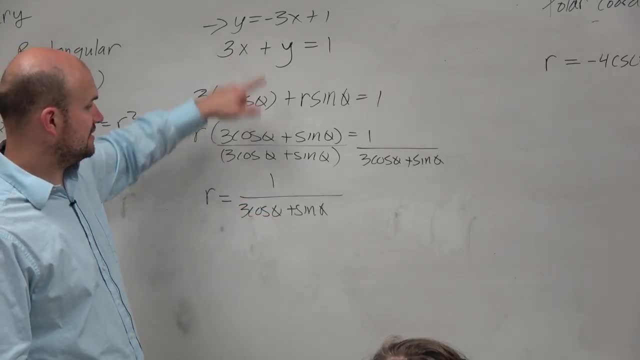 This is just in polar form. That's rectangular, That's polar form, But that's the equation of line. I can give it to you at the beginning of the year and say, hey, what's that equation of You'd be like? eh, no idea. 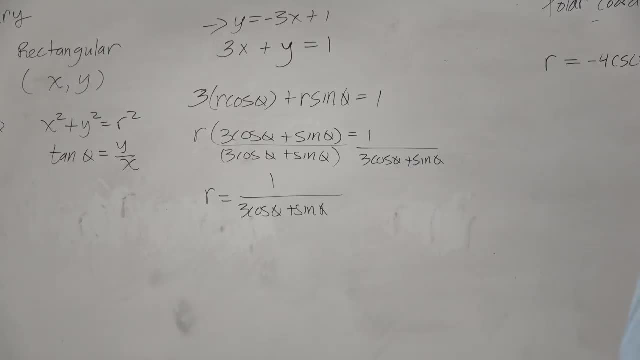 Mr McElogan, Yes, Can we have Abigail to the main office, Osterman check out, please. OK, Thank you. 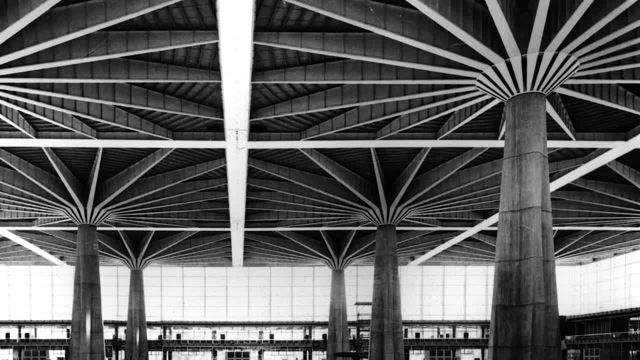 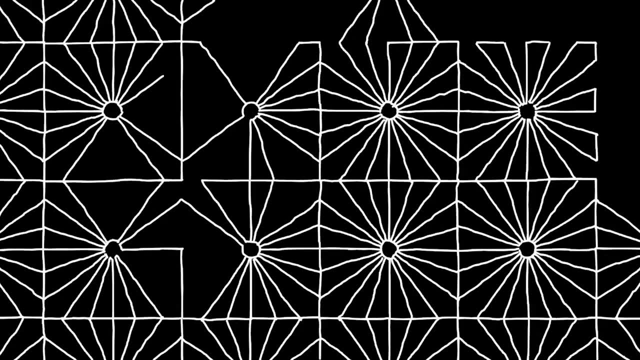 It is pretty safe to say that geometry is important to architecture. There's clearly some advanced geometric operations going on in some of architecture's complicated shapes or at the very least in the calculation of structural forces. And then there's all those shows on PBS and the Discovery Channel which claim to uncover secret messages encoded in